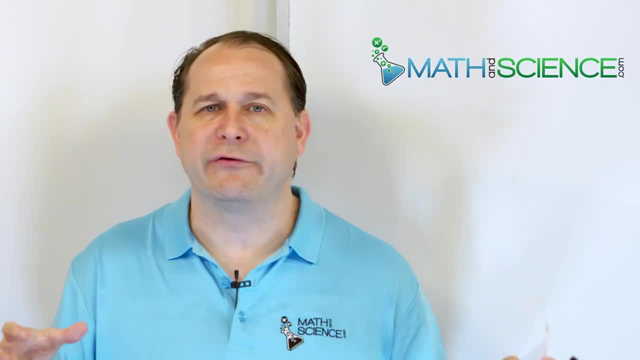 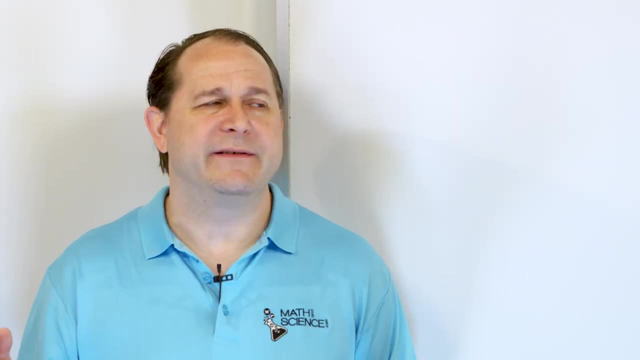 since antiquity, people have been looking at what the universe is made of around us and trying to figure out what the universe is actually made of. And so we would do thought experiments, you know, thousands of years ago, the ancient Greeks and so on, to try to figure out, well, what would happen. 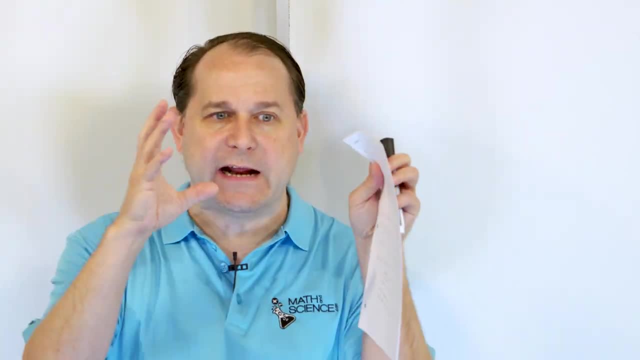 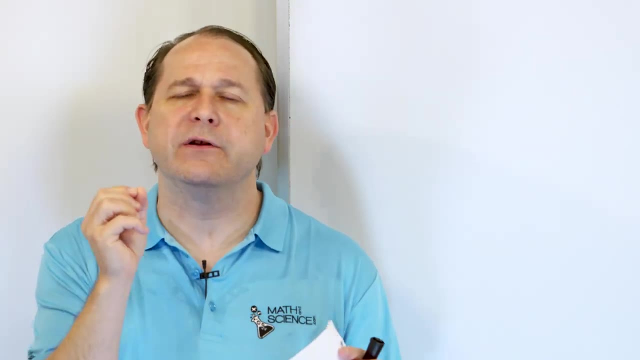 if I take in a block of matter and I cut it in half, and then I take that result and I cut it in half, and I keep cutting it in half over and, over and over again, will I eventually get to a fundamental building block of matter? And the prevailing idea at the time was that, yes, you. 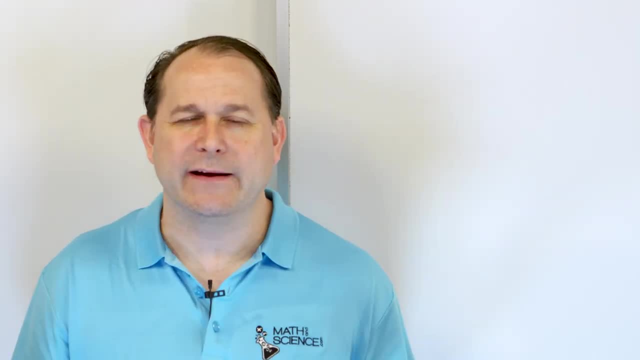